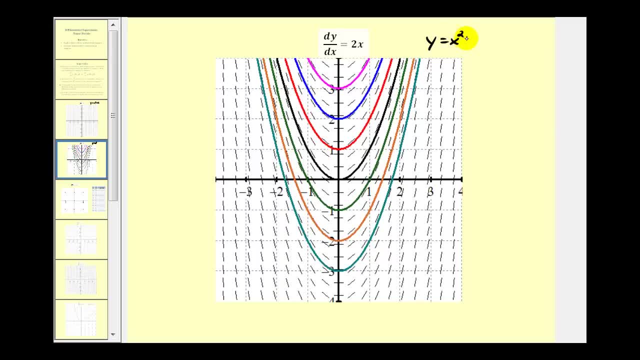 again in the form of: y equals x squared plus c. When we do this, you can see that these segments would represent the slope of the tangent lines at the given values of x to each of these functions. Now let's make our own slope field from the very beginning. 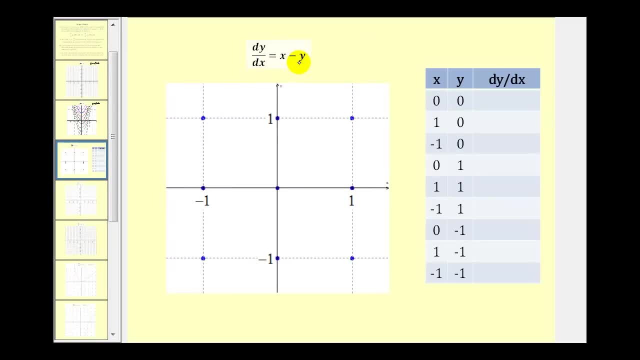 To make a slope field for dy dx equals x minus y. we'll make a table of values And notice for this differential equation. to find the slope of the tangent lines we need both an x and y coordinate. So for a small sample we'll select these nine points to determine dy dx. 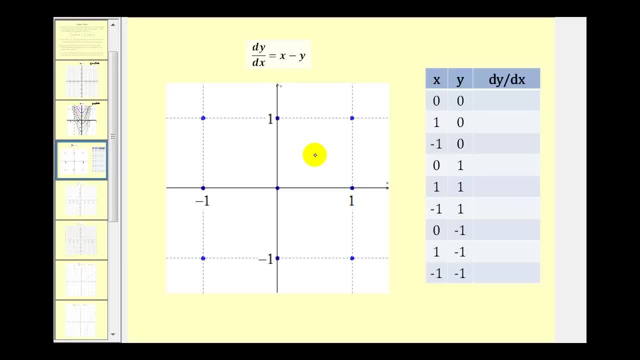 and then sketch a small segment to represent the slope of the tangent line. Again, dy dx is equal to x minus y. So at the point 0, 0 of the origin, dy dx is going to be equal to 0 minus 0 or 0.. 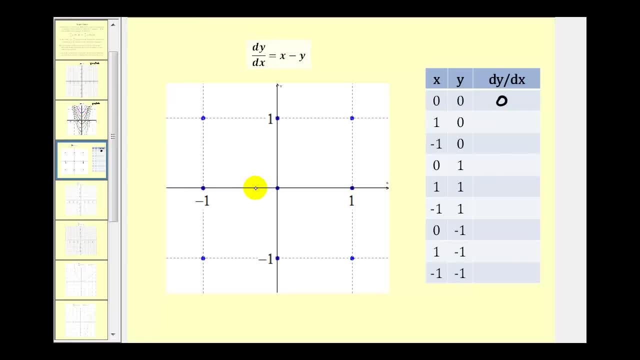 So at the origin we make a small segment with a slope of 0, which would look something like this: At the point 1, 0 of this point here, dy dx is 1 minus 0, which is 1.. 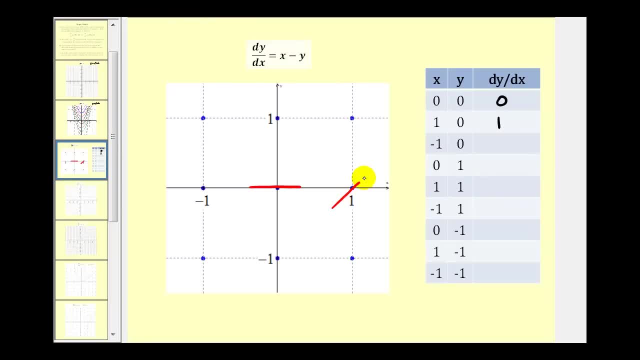 So we make a small segment here with a slope of 1, that would look something like this: At the point negative 1, 0, dy dx is negative 1 minus 0 or negative 1.. So at this point here we have a segment with a slope of negative 1,. 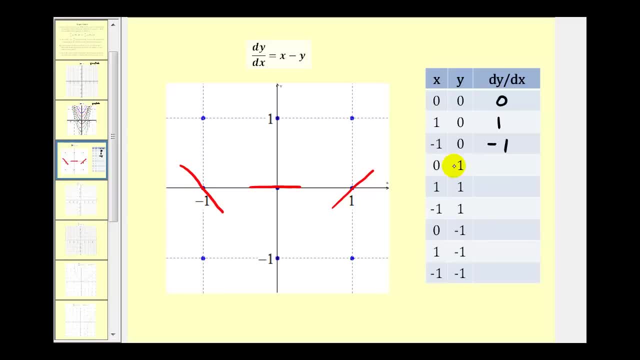 maybe something like this: At the point 0, 1, we would have 0 minus 1, which is negative 1.. So at the point 0, 1 of this point here, we'll make a small segment with a slope of negative 1,. 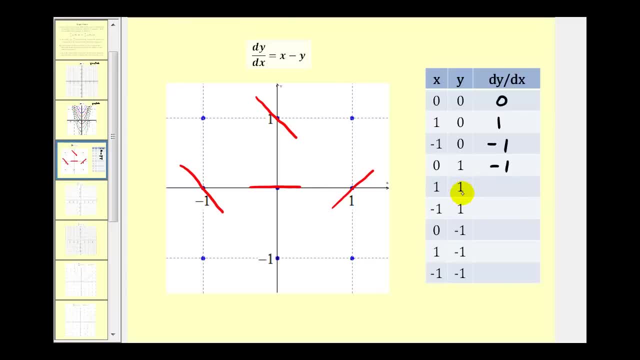 something like this: At the point 1, 1, since 1 minus 1 is equal to 0, dy dx is 0 at this point here. So we make a horizontal line or horizontal segment here, And so on. So negative 1 minus 1 is negative 2.. 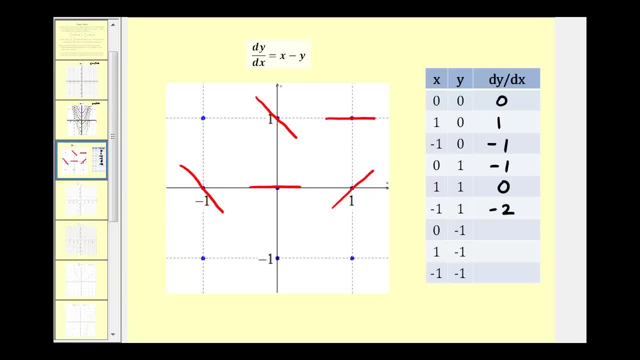 So at negative 1, 1 of this point here we'll make a segment with a slope- negative 2, maybe something like this: At the point 0, negative 1, we'd have 0 minus negative 1, which becomes 0 plus 1.. 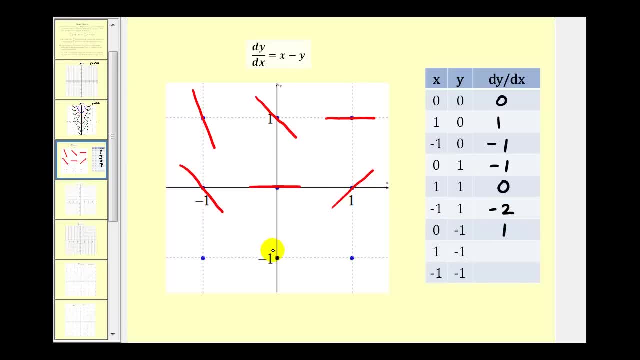 So positive 1. The point 0, negative 1 is here Small segment with a slope 1. At the point 1, negative 1, we'd have 1 minus negative 1 for dy dx, which is positive 2.. 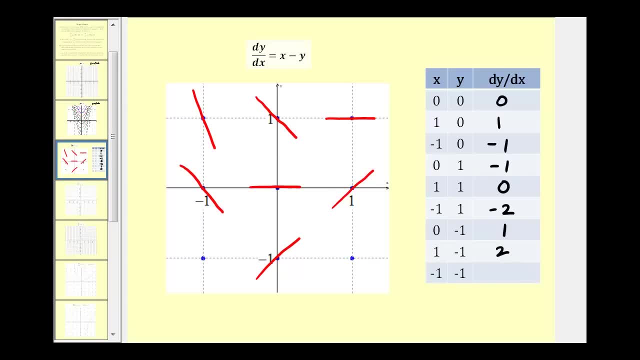 So at the point 1, negative 1. here we'll make a segment with a slope 2, maybe something like this, And then for the last point we'd have negative 1 minus negative 1, which would be 0.. 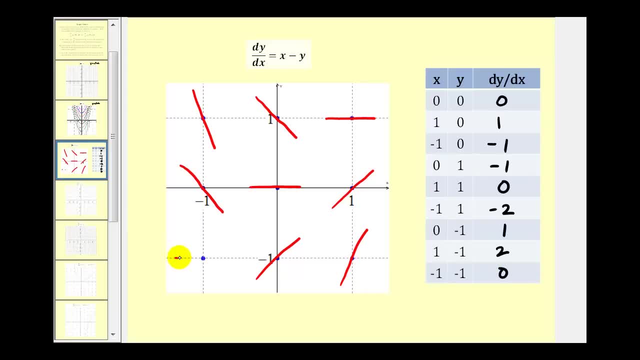 So at this point here we make a segment with a slope 0.. So here's a small sample of how we create a segment with a slope 0. We create a slope field And you can see it's fairly time consuming And that's why we often use technology to sketch slope fields. 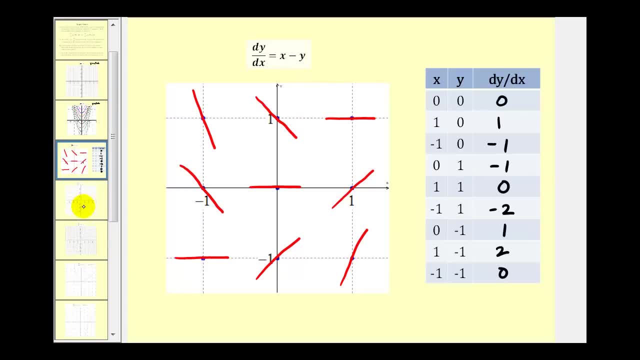 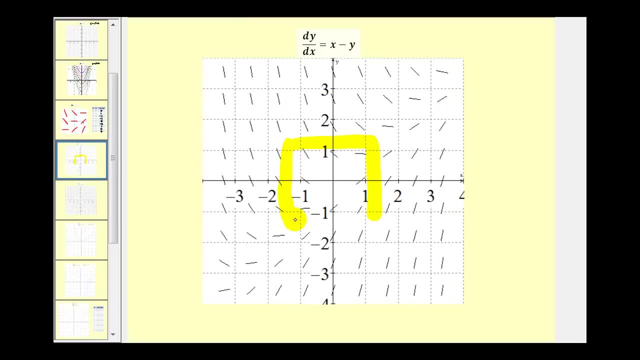 Now let's get a better picture of this slope field using technology. Again, on the previous screen we just sketched this much of the slope field, But now, with technology, we've expanded it to include from negative 4 to positive 4,. 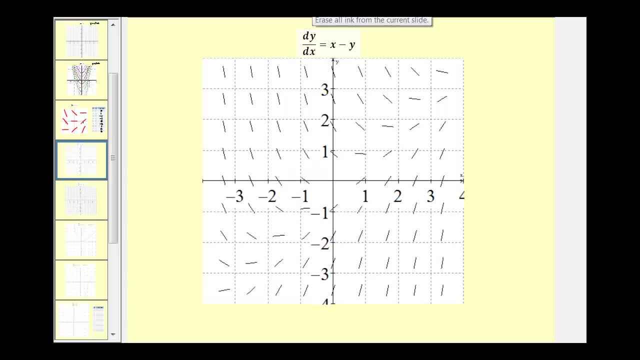 both along the x and y axis. Again, this represents the general solution to a function that would satisfy this differential equation, where each segment represents the slope of the tangent line at that given point, And with technology we can increase the number of segments plotted on a given interval. 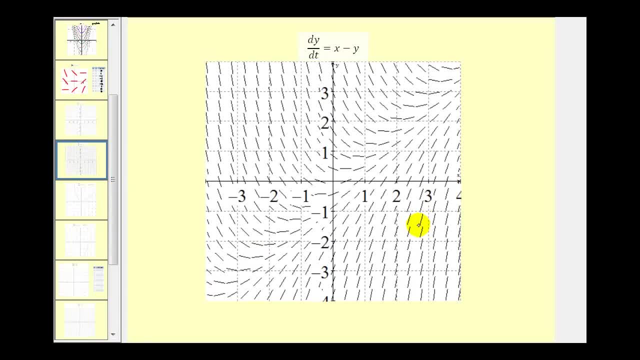 So here's the same slope field, but now we're sketching more and more segments on the same intervals, And again this represents the family of solutions to this differential equation. But for example, if we were given additional information, for example, if we were told that the solution contained the point 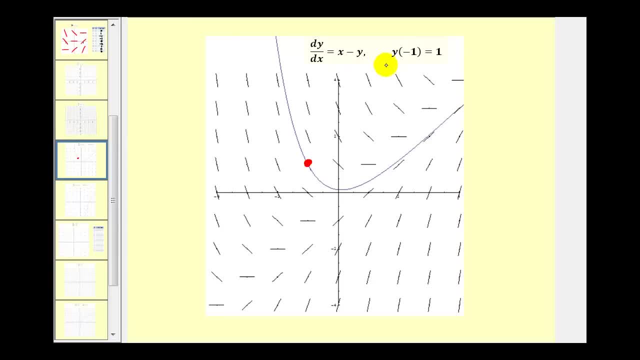 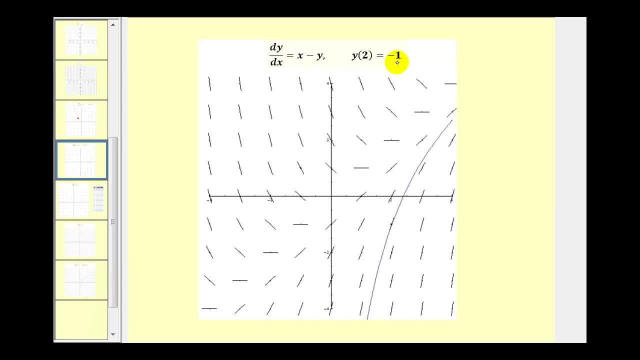 negative 1, 1, or that y of negative 1 was equal to 1,, then this would be the only solution to this differential equation and this function would be called the particular solution to this differential equation. For another example, if we were told that y of 2 equals negative 1,, 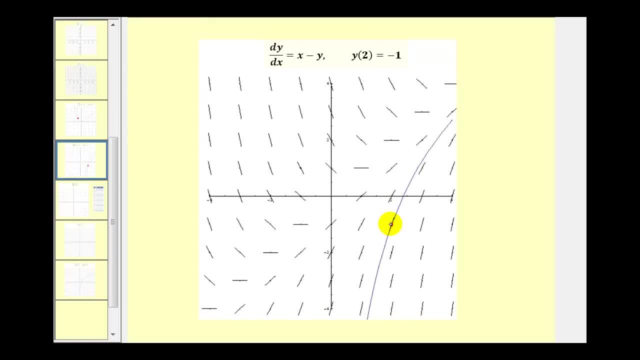 or the function contains the point 2, negative 1 at this point here, then this would be the graph of the particular solution graphed over the slope field. At this point, let's take a look at the difference between a slope field and a direction field. 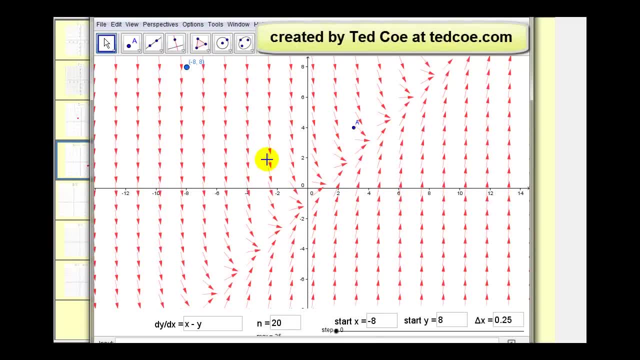 Again, the only difference is that the small segments have arrows in the direction of the increasing value of t or, in this case, x, And again, if we knew the function contained this point here, then we could graph the particular solution by following the slope field. 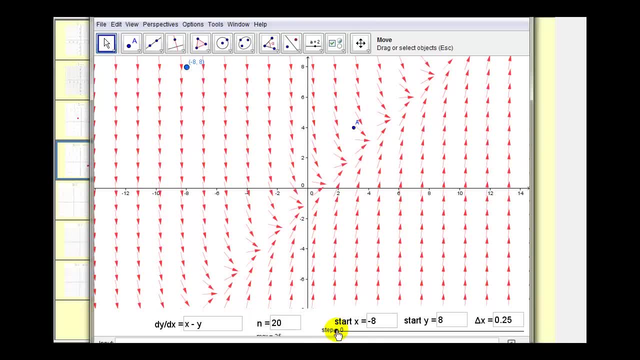 or, in this case, the direction field. The particular solution would look like this And you can see how it follows the direction of the direction field. Notice, as I move this point, which we're given as being on the solution, it is going to change the graph of the solution. 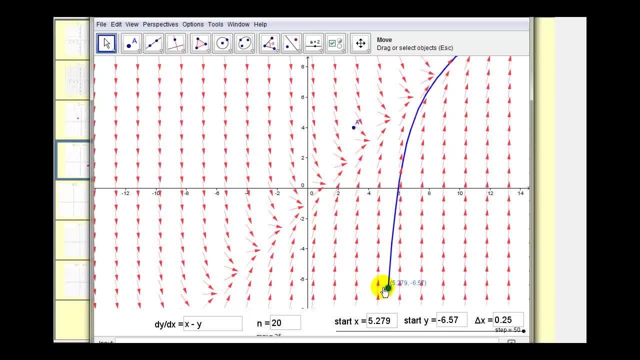 Again, if we're given an initial condition or a point on the solution, we can find the particular solution rather than just graphing the slope or direction field to represent the general solutions to the differential equation. Let's go ahead and take a look at one more slope field. 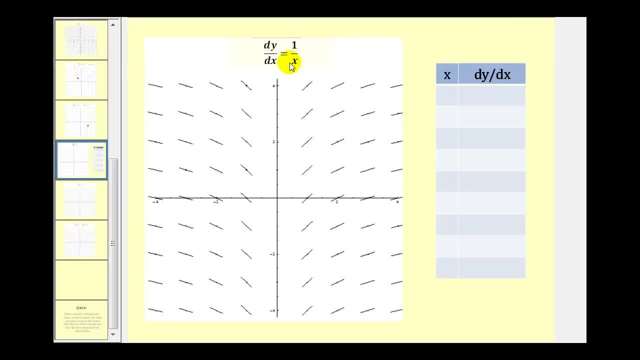 Here we have dy. dx equals 1 divided by x. Notice, in this case we can find the slope of the tangent line by just using the x coordinates rather than both the x and y coordinates. So if we use 3,, 2,, 1,, 0,. 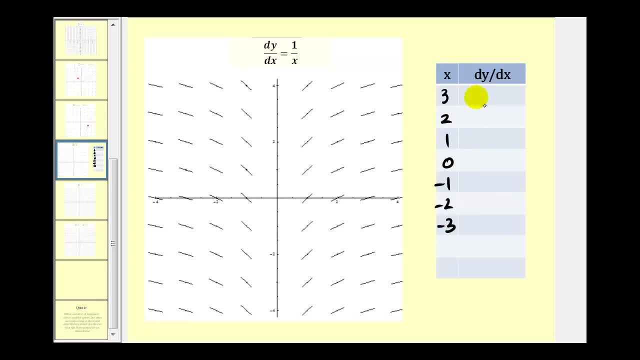 negative 1, negative 2, negative 3, dy dx is just going to be the reciprocal or 1 divided by x. So at x equals 3, dy dx is 1 third. At x equals 2, it's 1 half. 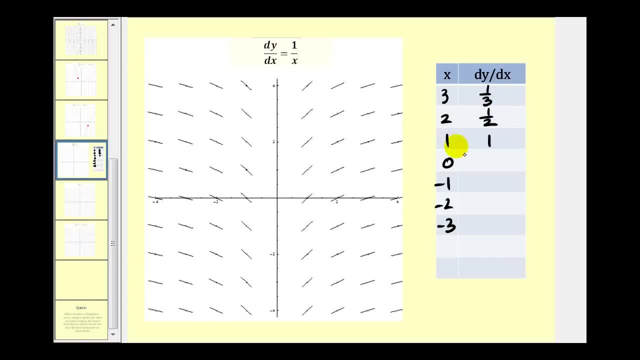 At x equals 1, it's 1 divided by 1, or 1.. At 0,, it's undefined, because we have division by 0.. At negative 1, it's negative 1.. At negative 2, it's negative 1 half. 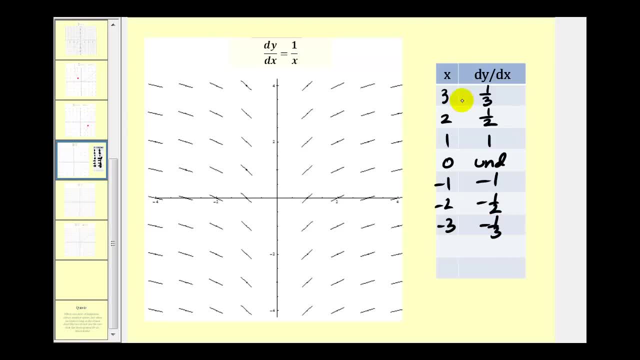 At negative 3,, it's negative 1 third. If we take a look at x equals 3, right here, all these segments have a slope of 1 third. At x equals 2, all these segments have a slope of 1 half.